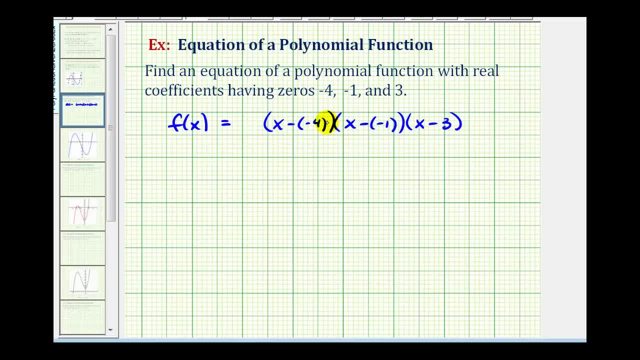 but since we don't have any fractions, we'll go ahead and let a equal one. So now we're going to simplify our binomial factors and then find this product: So f of x is going to be equal to: we have a factor of x plus four, a factor of. 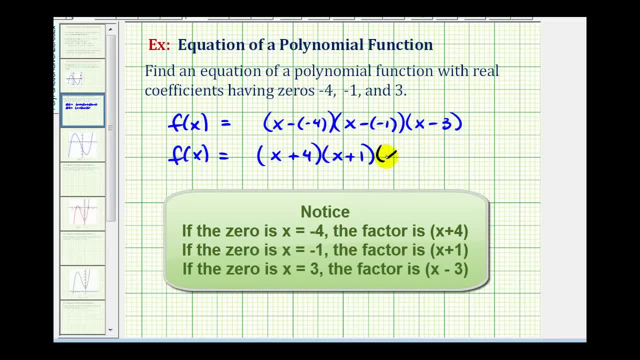 x plus one and a factor of x minus three. Now to multiply this out. there's no shortcut. We can only multiply two binomials at a time. So we'll multiply the quantity x plus four times the quantity x plus one, so we'll have four products. 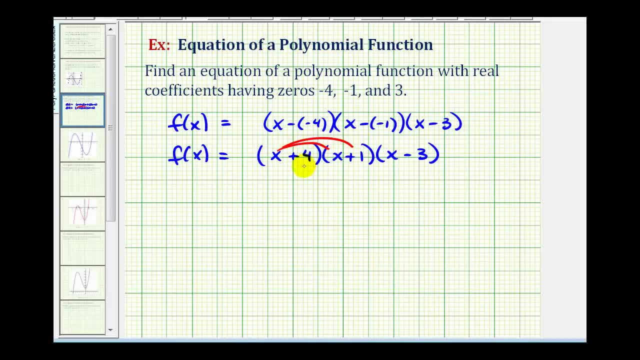 One, two, three, four. So we'll have f of x equals x times x, that's x squared X times one, that's one x. And then we have four times x, that's four x. One x plus four x is five x. 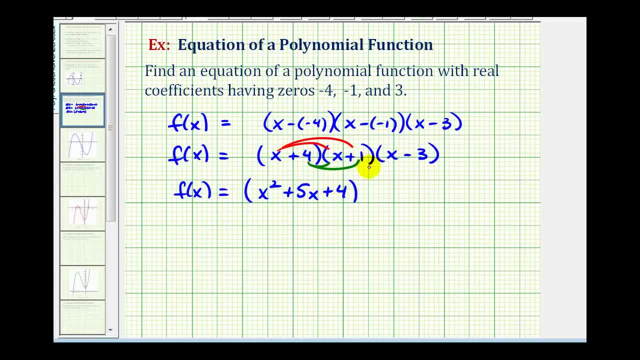 And four times one is positive four. So we have this trinomial times, the binomial x minus three. Multiplying these two, we'll have six products: One, two, three, four, five and six. So we'll have f of x. 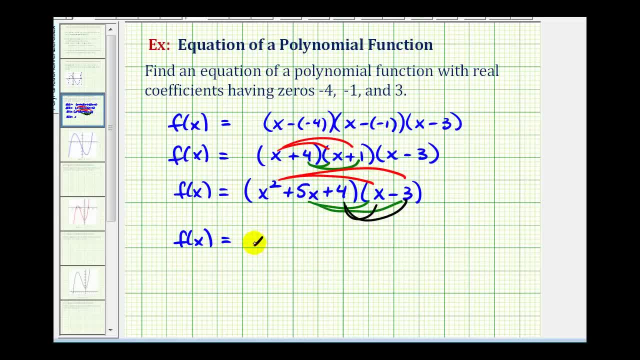 equals x to the second times x, that's x to the third, X to the second times negative three, that's negative three x squared, or minus three x squared. Then we'll have five x times x, that's five x squared. so plus five x squared. 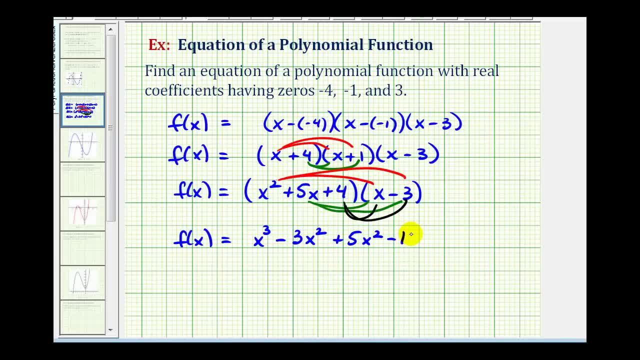 Five x times negative three, that's negative fifteen x or minus fifteen x. Then we have four times x, that's plus four x. Then we have four times negative three, that's negative twelve. so we have minus twelve. Last step: we want to combine our like terms. 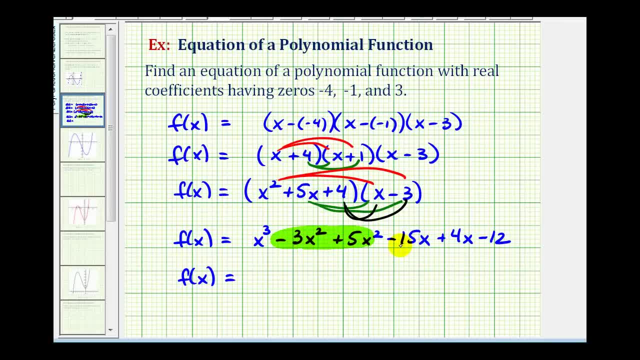 So we have two x squared terms and we have two x terms, So one possible function with these zeros would be: x cubed negative. three x squared plus five x squared, that's positive two x squared. so plus two x squared, Negative. fifteen x plus four x is negative eleven x or minus eleven x. 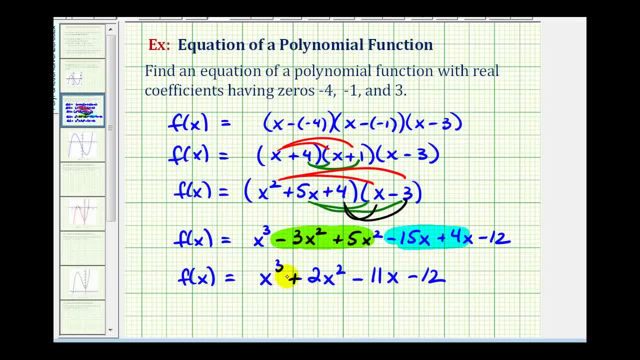 and then minus twelve. So again, this polynomial function, which is also a cubic function because it's degree three, would have the real zeros of negative four, negative one and positive three. And to verify this, since these are real zeros, we can graph this function. 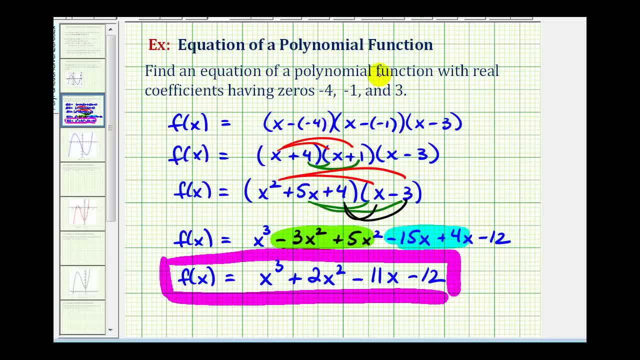 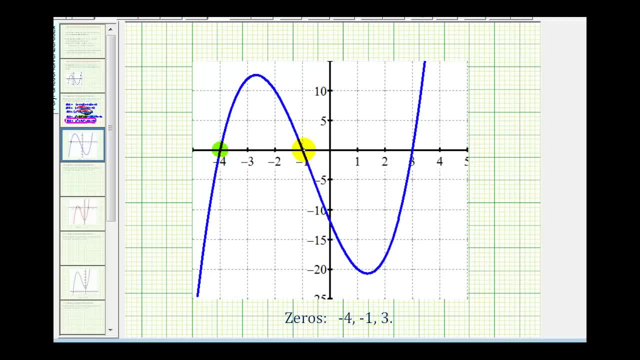 and verify. these would be the x intercepts of the graph. So here's a graph of the function that we just found. Notice how we have the x intercept of negative four, negative one and positive three, which verifies our work. Okay, I hope you found this helpful. 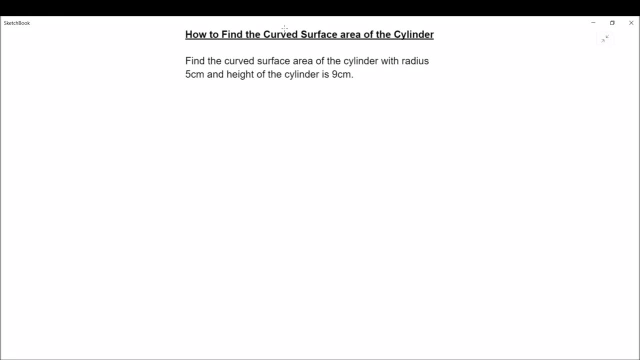 Hello everyone, in this video we are going to learn how to find the curved surface area of the cylinder using the formula. The formula we are going to use is: curved surface area is equal to 2 times pi times r times h, where r is the radius of the cylinder and h is the height of the cylinder. 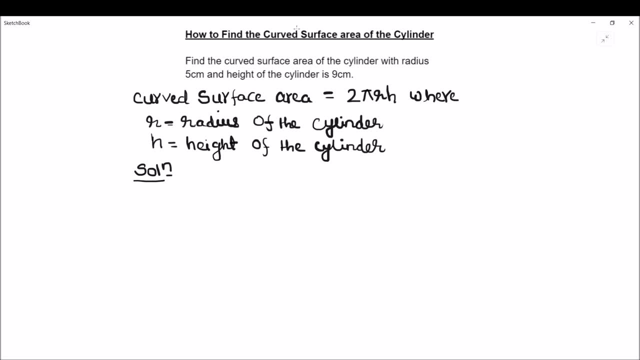 So let us read our question. The question is: find the curved surface area of the cylinder with radius 5 centimeter and height of the cylinder is 9 centimeter. So we have been given radius as 5 centimeter and the height of the cylinder is given as 9 centimeters. 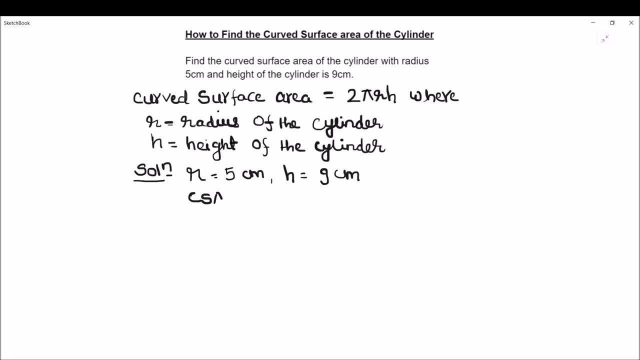 So let us substitute the values in our formula: curve surface area. I am writing it: csa is equal to 2 pi. rh 2 times pi is 22 divided by c. Radius of the cylinder is given as 5 centimeters and height is given as 9 centimeters. 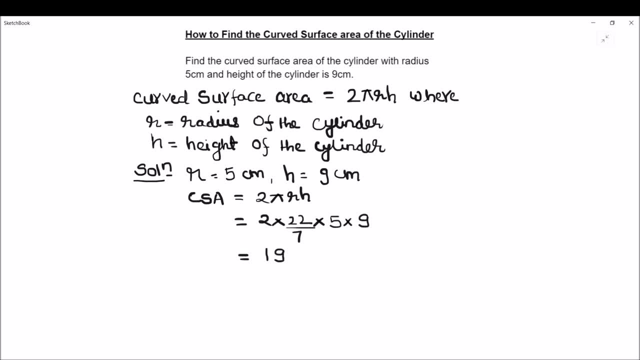 So, after calculating, we will be getting 1980 square centimeters divided by 7, which comes out to be 282.85 square centimeters. The curved surface area of the given cylinder is hundred and eighty two point eight five square centimeters. so this is how, by 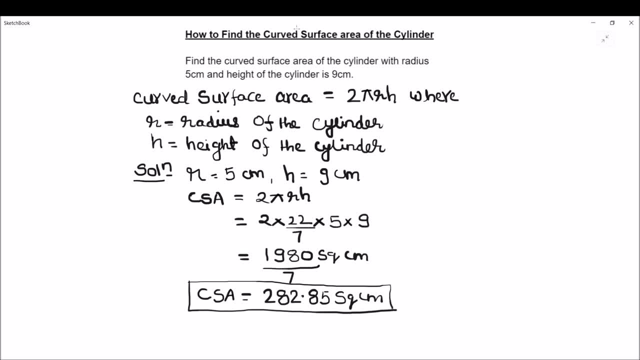 using the formula, you can find the curved surface area of any cylinder easily. I hope this video is helpful to you. if you like to see more videos on surface area and volume, you can check out my playlist, which is in the description. if you like the video, please hit the like button and subscribe to my